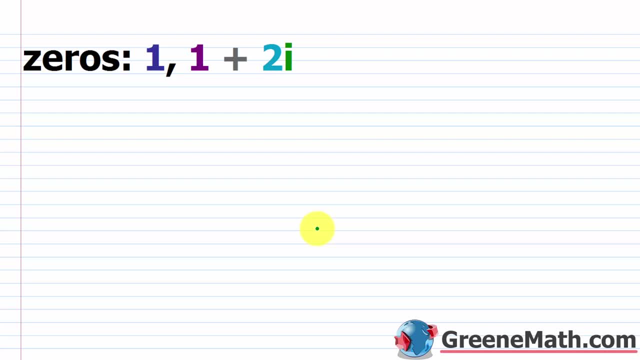 this in the last lesson. Basically, what we're going to do is we're going to find a polynomial of least degree having only real coefficients and zeros that meet this criteria. So the zeros given are one and one plus two i. So we know that this guy right here, this one, that's just a. 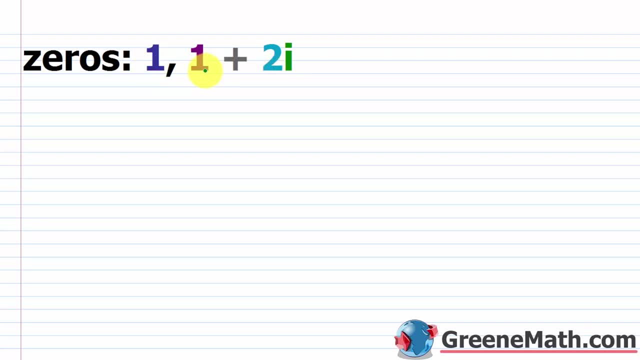 regular zero. We've been working with that forever. But when we get to the next one, we're going to get this complex zero one plus two i. well, we know that it's going to have its conjugate as a zero as well, So we can go ahead and write in here that another zero would be one minus two i Again. 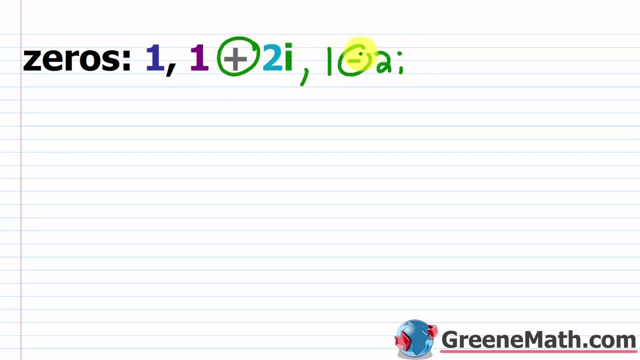 the one stays the same. the two, i stays the same. just change the sign to get the conjugate. That's all you're doing. So now, if I want to write out my polynomial function, remember the form: It's: f of x is equal to: it's a times you have your x minus k sub one, times your x minus k sub two. 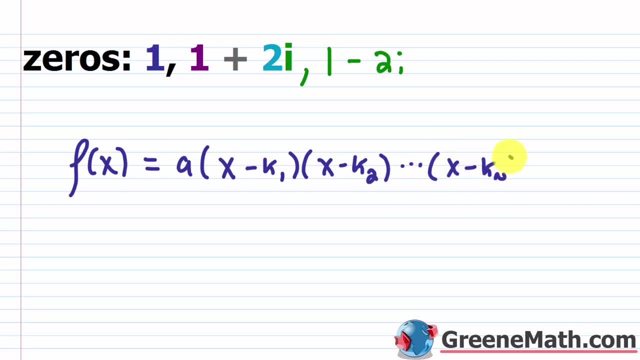 and then you keep going and then you have your x minus k sub n. So in each case it's x minus whatever the zero is. So in this one I'd say x minus one, And then for these it's going to be: 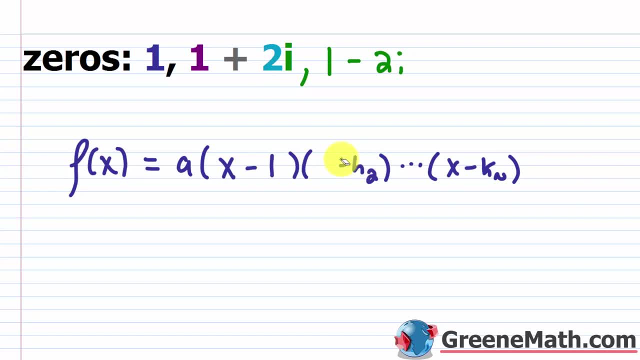 a little bit more complicated because I'm subtracting away a complex number. So let me just kind of write this off here And I'll say that this is x minus. I'll put it in parentheses: one plus two i, And then let me close that and I'll do x minus. now I'm going to do one, let me slide. 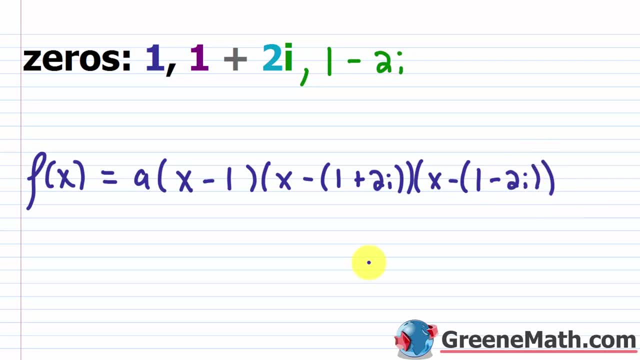 around And now we'll have minus two. i go ahead and close that off. Okay, now, in this particular case you're not given any information. I know in the last section we were given a point and then we could figure out what a is. So here a is just going to be one, so you can just erase it or put. 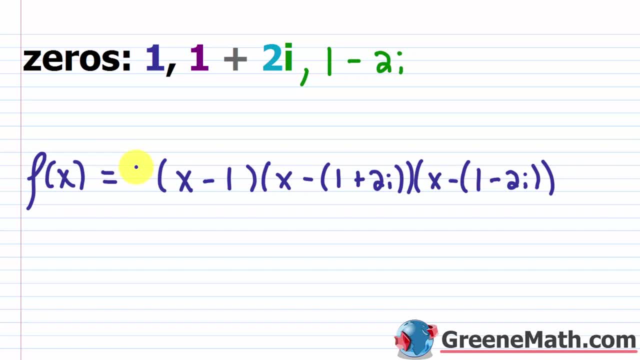 a one there, And what happens is we're just going to go through and simplify this. it's going to take a little bit of time because it is quite tedious, But we'll have our polynomial function And it's a good exercise to kind of practice working with these complex numbers. Okay, so 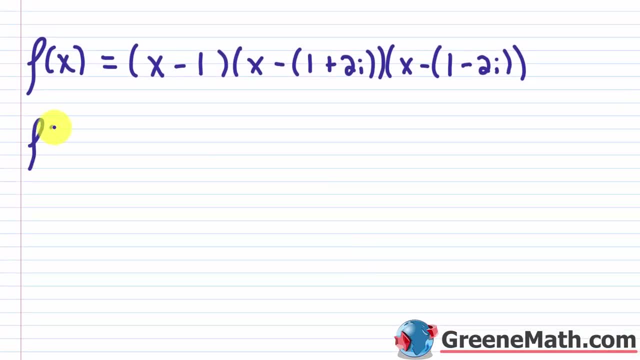 let's go through and start simplifying. So I'll say f of x is equal to- I'm going to leave this for last. So I'm going to have x minus one outside of, and I'll just put some brackets here And the way. 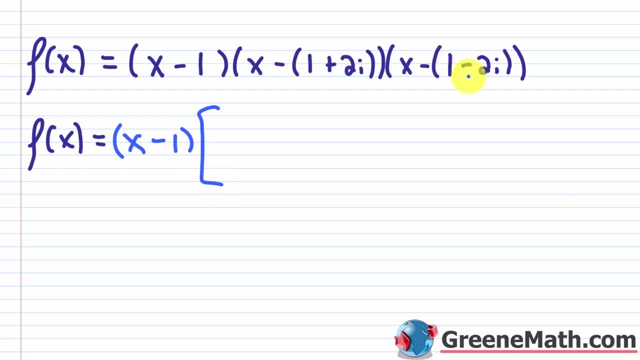 I'm going to do this is I'm going to do FOIL with these guys as they are. Okay, so I'm going to treat this as the first term and this as the second term in each polynomial. So this is your first term and this is going to be your second term. Okay, so I'm going to say that I have what First. 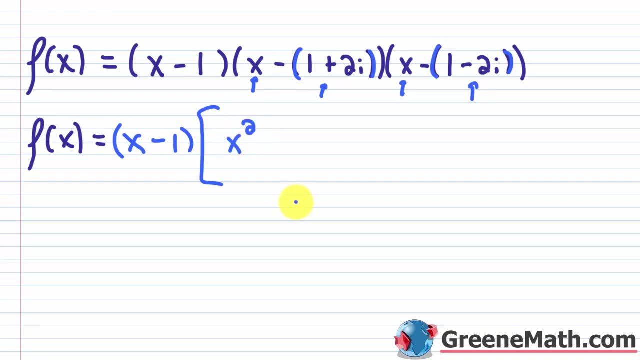 times x is x squared. And then my outer terms: I would have x times negative this guy, the one minus two i in parentheses, So remember the minus- and you have x times this quantity, one minus two i. Okay, And then continuing, and I'm probably not gonna be able to fit all this, But I'll try. 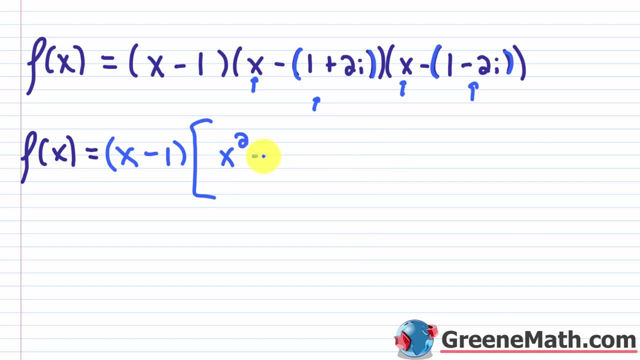 and see if we can squeeze it down. So let me erase this and put minus x times again one minus two. i is kind of scrunch that down a little bit. So when I go to my inside terms I'm going to have this negative times, this one plus two. i that quantity times. 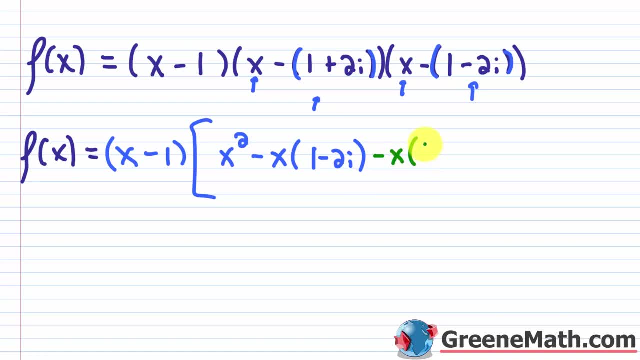 this x. So I'll have minus x times again this quantity: one plus two i. And then, for the last terms, I have this guy times this guy. Now it's negative, times negative, So I know it's going to be a positive, Okay, And then what I want to do is say that I have what: One plus two i times one. 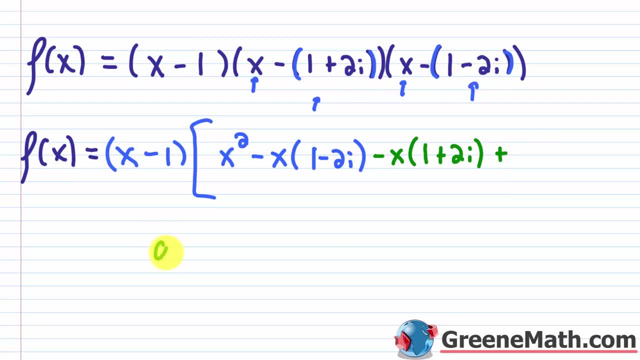 minus two. i Well, I know my formula for that, Remember, if you have a plus b times a minus b, this is a squared minus b squared. Okay, So in this particular case, I'm just going to write this down here because I'm just going to run out of room. 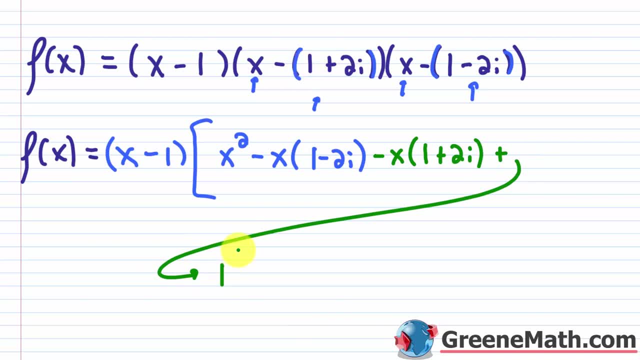 I'm going to say that I have what The first guy squared, So one squared, which is one minus the second guy squared. So if I take two and squared, I get four. If I take i and square it, remember i squared, by definition, is negative one, So this would be negative one. So really, 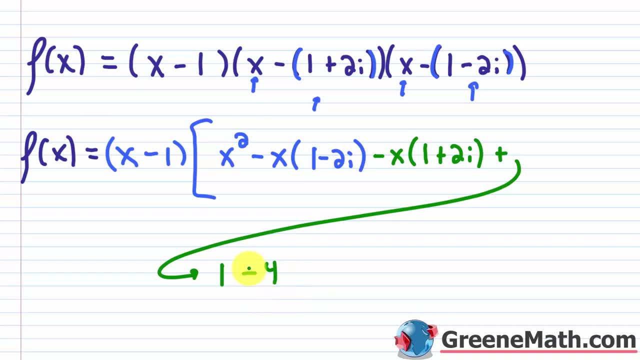 you have negative four times negative, one which is positive four. So one plus four is just going to be five, So I can write this as five here, And that allows me to fit everything on my screen. Okay, So now we're going to simplify. Let me scroll down and get some room going and see where we are. 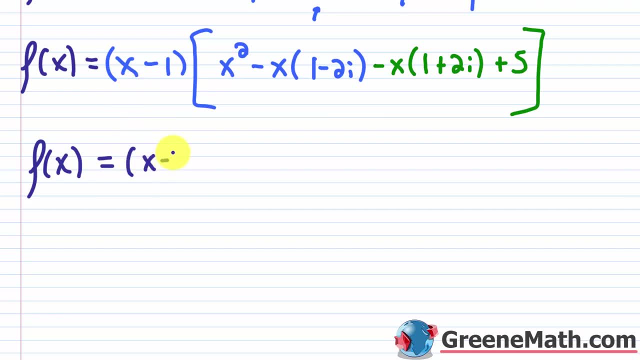 So we have f of x equals. I've still got this x minus one out in front And inside. I'm just going to see what I can do to simplify, So let me put my brackets here. So I have my x squared And then I 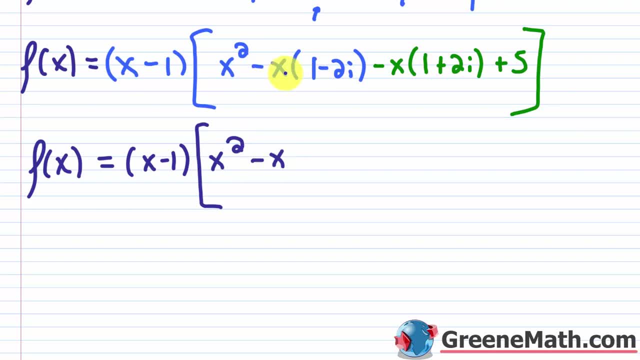 have my negative x times one, which is just minus x, And then negative x times negative two. i would be two i x. Then, moving down here, I have negative x times one, which is minus x, And then negative x times two. i is going to be negative two i x. And then, lastly, I have my plus five. Okay, so what we? 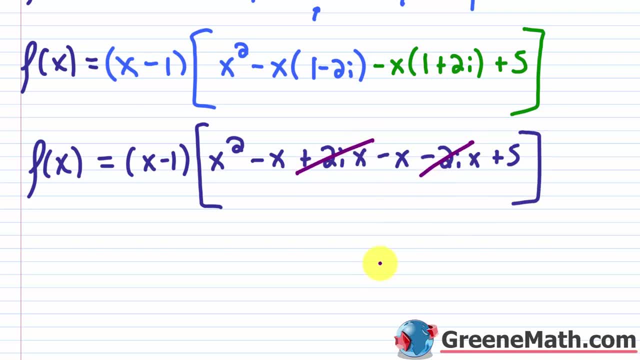 see now is that this will cancel with this, And negative x minus another x would be negative two x. So let's go ahead and write that we'd have f of x equals the quantity x minus one times. I'll have x squared Again. negative x times. negative two i x. So that's going to be negative x times. 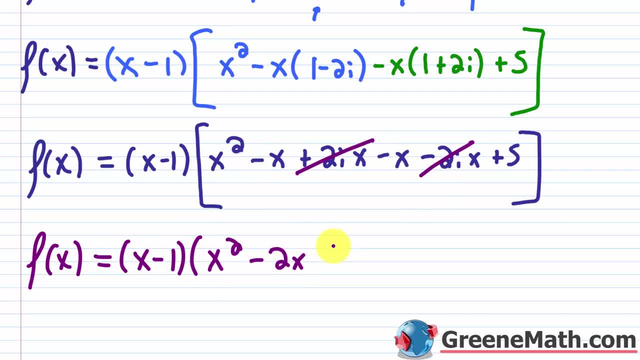 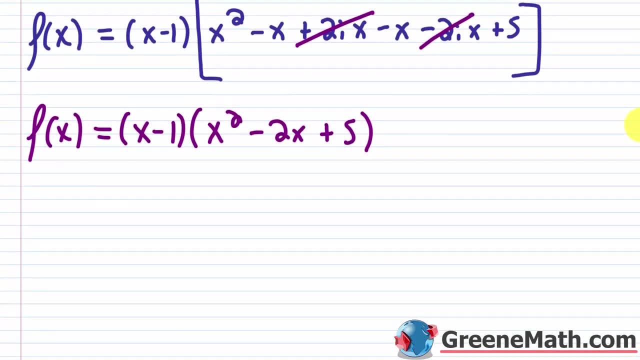 x minus x is minus two x, And then we're going to have plus five. So starting to look pretty good. Let's scroll down a little bit. I know this is tedious, but you have to do some examples of these. So we'll have f of x is equal to. I'll go through and multiply x by everything, So x times. 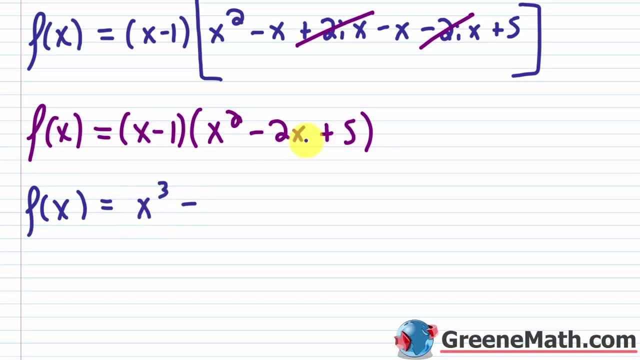 x squared is x cubed, And then minus x times two x is two x squared. And then plus we have five times x, which is five x, And then I have a negative one times everything. So basically, I'm just going to choose negative one times everything, And then I'm just going to choose. 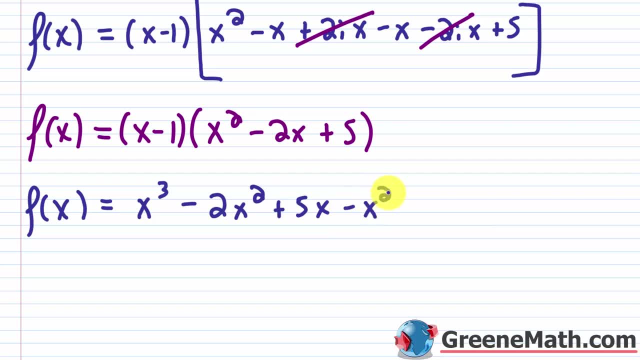 the sign of everything here. So I would have minus x squared, And then I would have plus two x, And then I would have minus five. Okay, so let's continue Now. all we have to do is just combine like terms. So x cubed. nothing to combine with that I have. let me get some room going here. 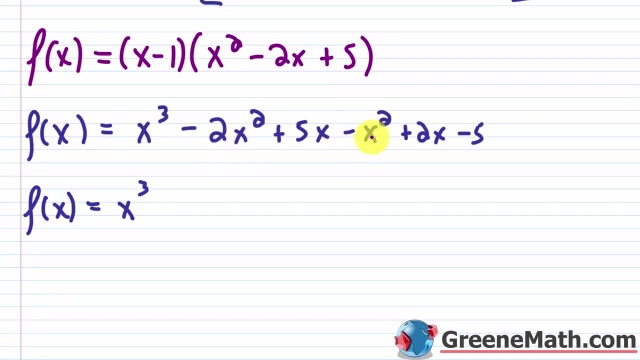 I have negative two x squared and minus x squared, So that would be negative three x squared. I have five x and two x, So that would be plus seven x, And then I have minus five, So we end up with our polynomial function. f of x equals x cubed, minus three x squared, plus seven x, minus five. All right, 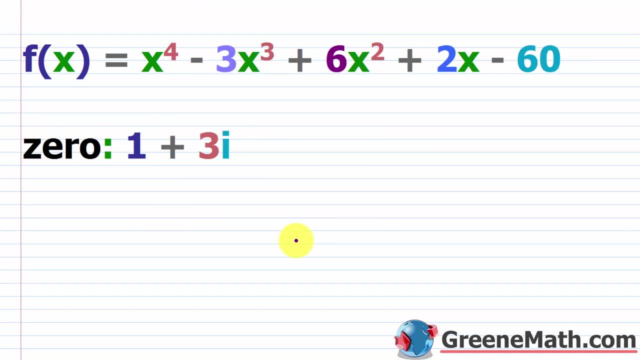 the next type of problem you're going to see is also pretty tedious. So suppose you're given some polynomial function. let's say f of x equals x to the fourth power minus three, x cubed plus six, x squared, plus two, x minus 60. And they say: find all the zeros, and they give you a complex zero. 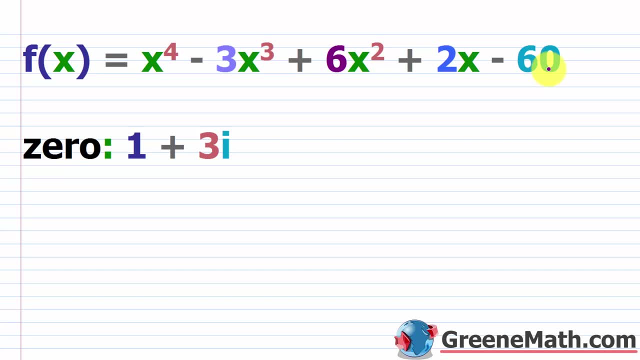 So let's think about what we know at this point. At this point, we know that the degree of the polynomial is four. So I know that I'm going to have four solutions- right, At most it would be four distinct solutions- But I know that I'm going to have four solutions, even if some of them are. 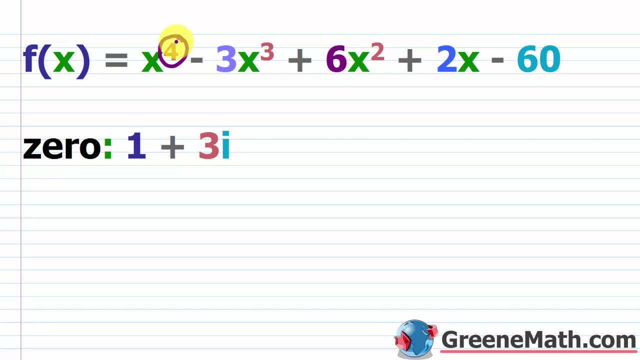 repeats: Okay. The other thing we know is that we're given a complex zero of one plus three, i, So there also has to be a zero of one minus three, i, because these come in conjugate pairs. Okay. So I know, if I have two zeros here, I can get this guy down to a quadratic. 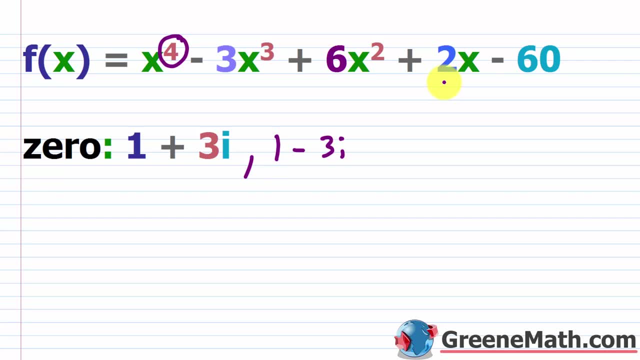 And at that point I can use the quadratic formula. Or, if I'm lucky, I can factor or complete the square, or whatever you want to use, It doesn't matter. We know that once we get it down to a quadratic we're good to go. So there's two ways that you could attack. 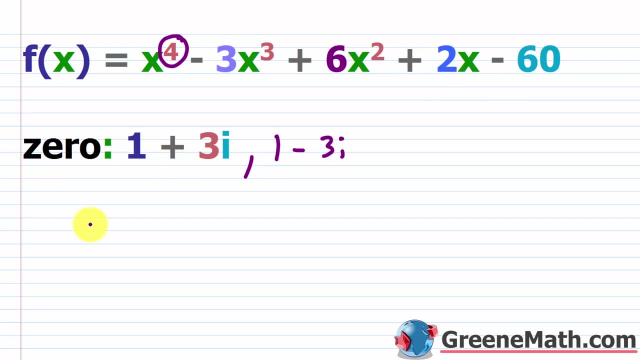 this problem. The first thing is you could write this out as x minus this, one plus three i. Okay, that's your factor, Let me make that clear. And then x minus you have your one minus three i. That's another factor. So you could multiply these two together, get that polynomial, Okay. 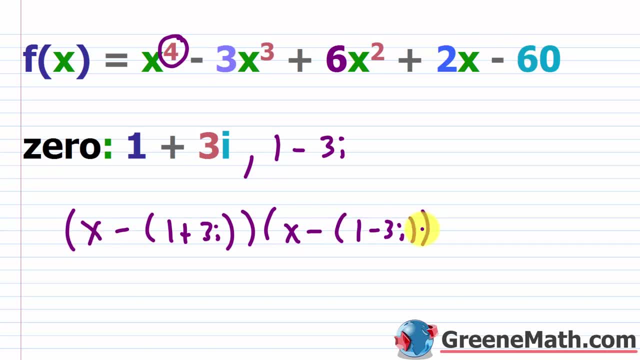 And then you could divide synthetically This guy by whatever that is, And that would give you two different quadratics that you could solve with the quadratic formula. So that's one way you could do it. Another way you can do it in the way 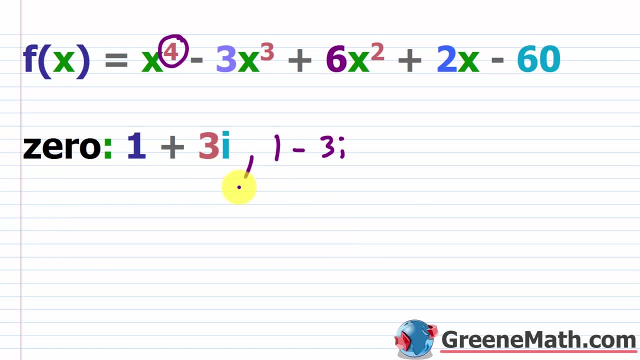 that I'm going to do. it probably would take a little bit longer. You can use synthetic division- Okay, With this guy and with this guy to get it down to a quadratic. So that's the way I'm going to do it, just to get a little practice of working with these guys and doing some synthetic division. 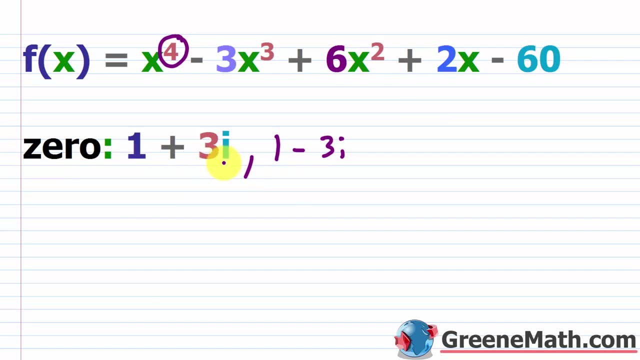 So I'm going to start with this one right here, Okay, And what I'm going to do is go one plus three i, And then over here I'm just going to take my coefficients. So, one negative three, we've got six, we've got two and we've got negative 60. And I made a little bit of a mistake. 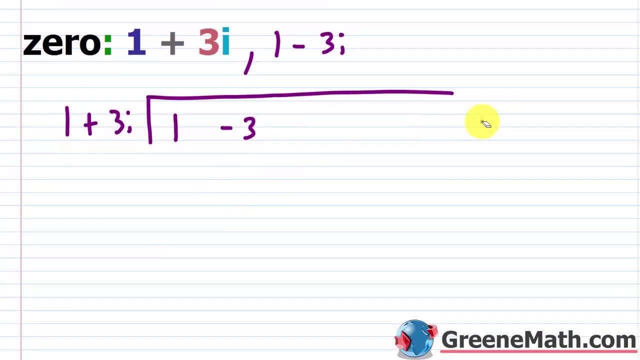 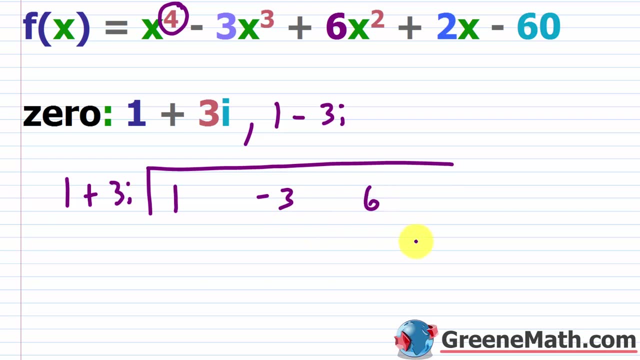 here, because when you work with this, you want to make sure you have a lot of room. So let me actually redo this. So let me come back up here and say that we have negative three. I'll push that over here, I'll push my six over here, my two over here and my negative 60 all the way over. 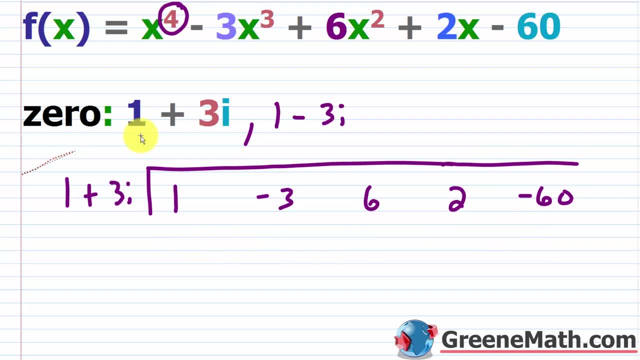 here You need room because these complex numbers they take up a lot of room. So I'm going to take a lot of space. So let me kind of move this down and then we'll be good to go. Okay, So let me put. 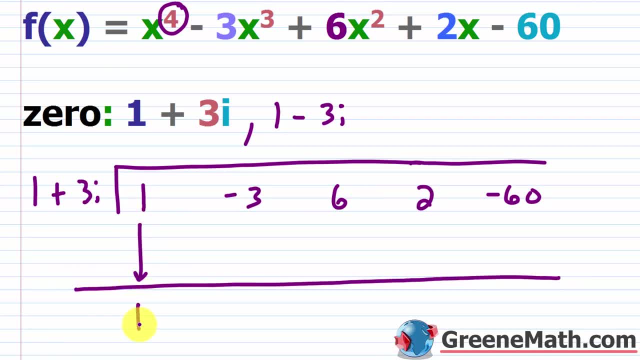 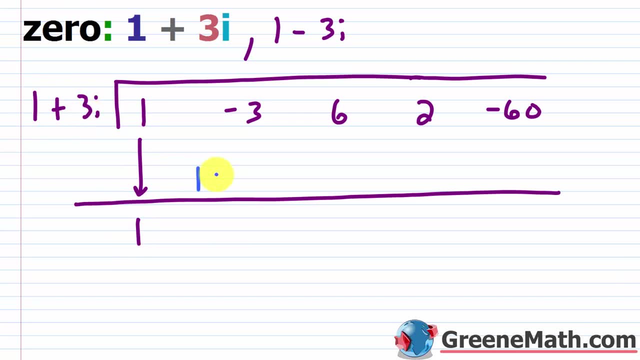 a bar down here. drop this down and we'll start. So we'll come back up in a minute, We'll go back and forth. So basically I dropped this down. One plus three i times one is one plus three i Okay. 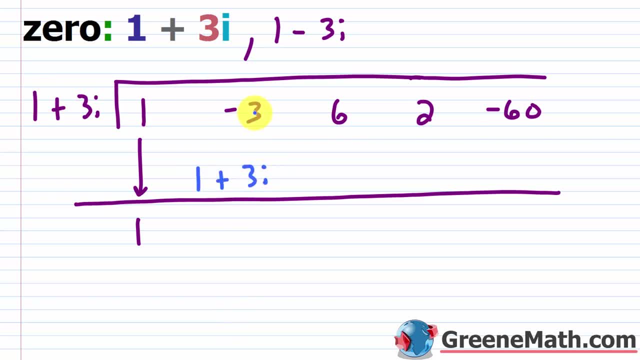 If I had negative three plus one plus three i, I just add the negative three and the positive one, which gives me negative two, And the plus three, i comes along for the ride. Okay. Now, where this gets tedious is that you have to multiply. now You multiply two complex numbers, You basically 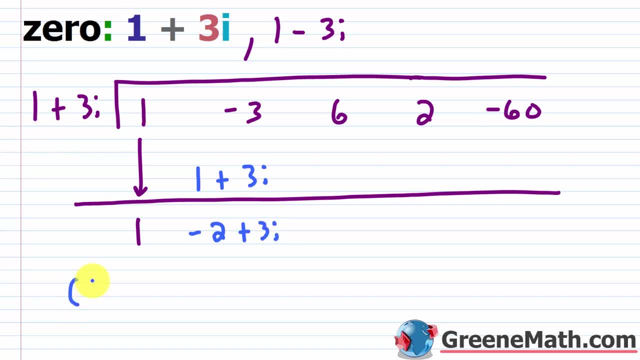 have to stop and do four. Okay, So we have this one plus three i times this negative two plus three i. Okay, So one times negative two is negative two. The outer would be one times three, i, which is plus three i. The inside would be three i times negative two, which is minus six i. And then the 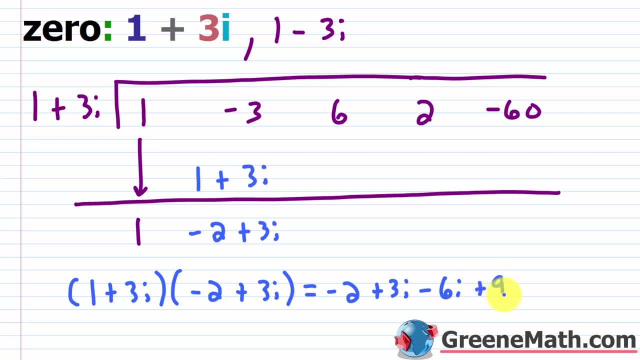 last three. i times three, i is nine. i squared. Now remember i squared is negative one, so you can really just say this is negative nine. Okay, So you have negative two minus nine, which is negative 11.. And then on top of that, you're going to have three, i minus six. i. 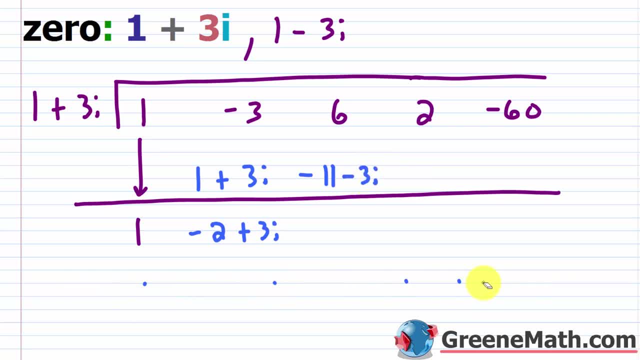 which is minus three i. Okay, So let's erase this. We don't need that scratch work anymore. And so if I said six plus negative 11 minus three, i, what is that? Again, you just work with the real parts. Six minus 11 is negative five. So this guy is going to be negative five minus three. i. 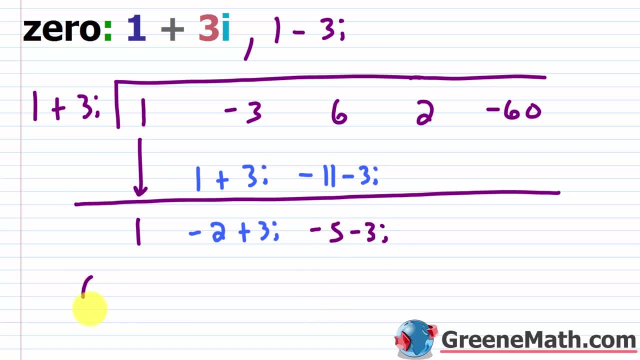 Okay. So here comes again the tedious part. We've got to multiply, So we have one plus three, i times you have negative five minus three, i. Okay. And then we're going to do one times negative five, That's negative five. We're going to do one times negative three, i. That's minus three, i. We're. 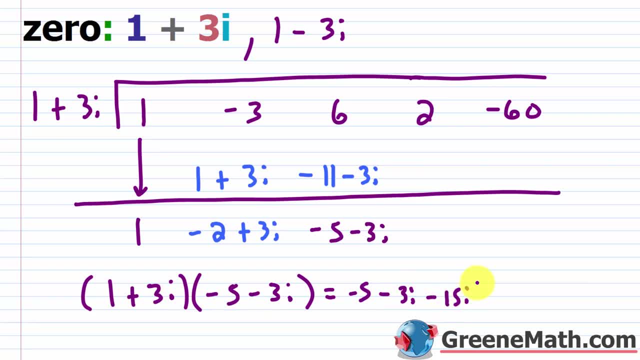 going to do three. i times negative five, That's minus 15 i. If you want to combine these at this point, it would be negative 18 i. Let's just go ahead and do that. And then, lastly, you have three i. 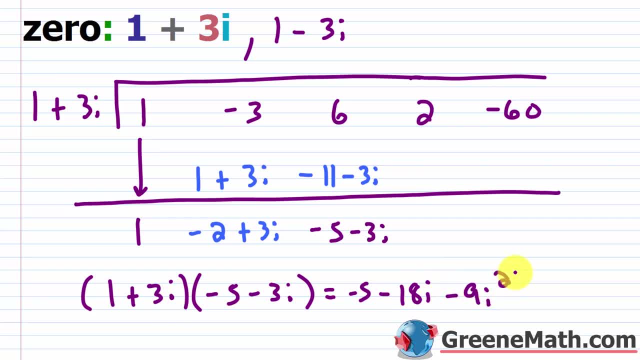 times negative three. i, So that's negative nine. i squared, But again i squared is negative one. So you're just going to change the sign of this to plus, So positive nine plus negative five. or you can think about this as nine minus five, That's just going to be four. So this would be. 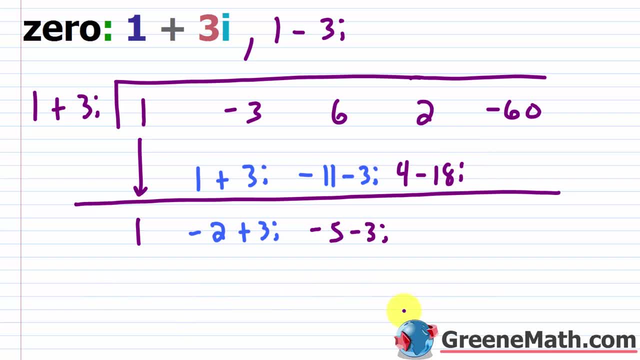 four minus 18 i. Okay, So now we want to add two plus four minus 18 i. Well, two plus four is six. That's all you're going to be able to do there. And then you bring the minus 18 i along for the. 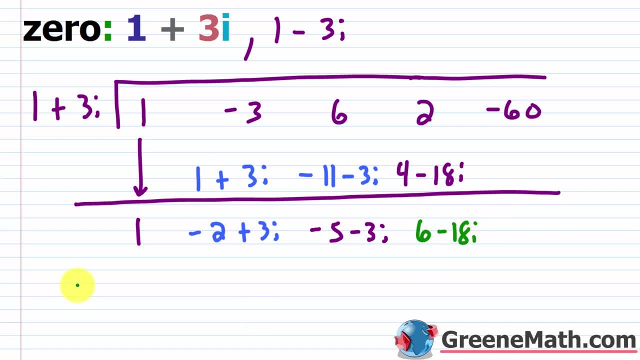 ride All right. Last multiplication: Again, I know this is going to be a little bit of a tedious, but we have one plus three, i times you've got your six minus 18 i. So one times six is six. And then I'm going to do my one times negative 18 i, which is minus 18 i, And then my 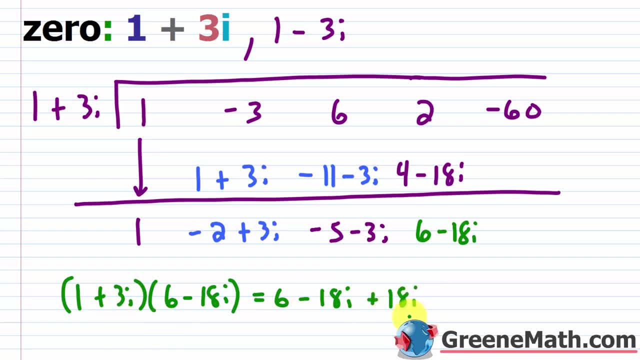 three i times six, which is plus 18 i. Okay. Then we have three i times negative 18 i. So we know that's a minus Three times 18 is 54.. And then you'd have i times i, which is: i squared, i squared. 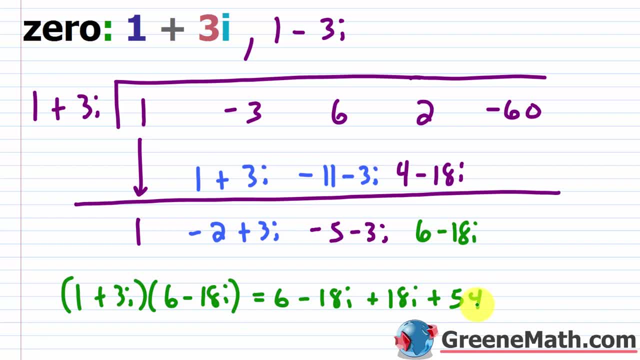 is negative one. So just change the sign So it's just plus 54.. 54 plus six is 60.. Okay, We know that negative 18 i and positive 18 i, those are going to cancel, So we're just left with 60.. We already knew this was a zero, So we knew we wouldn't have a remainder. 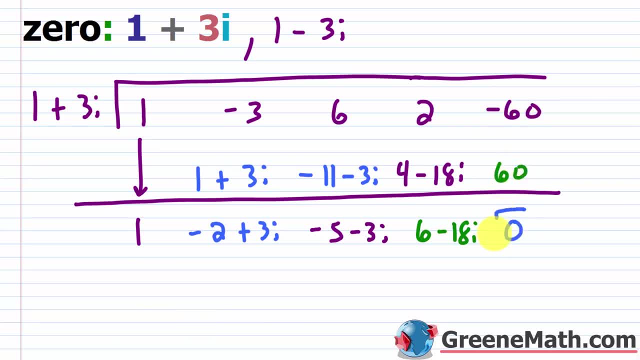 by definition. So we know negative 60 plus 60 is zero And that is what we would expect. right To have: no remainder or remainder of zero. Now, once we're done here, we already know that one plus three i is a zero. We don't need it. And we know that one minus three i is a zero, So we're going. 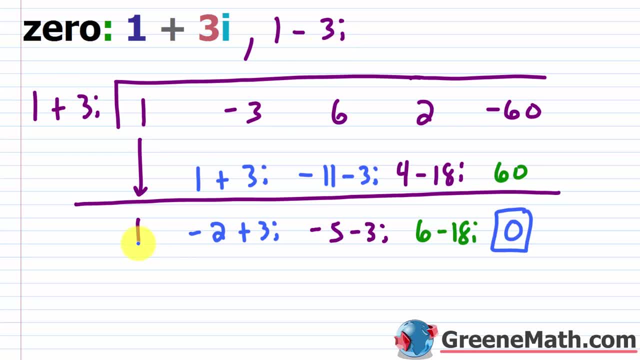 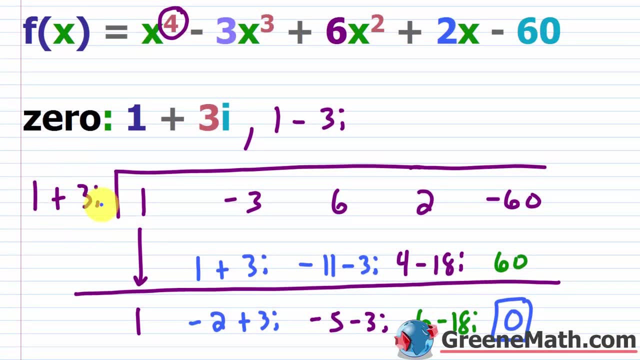 to use this information to further get this down. So remember, if you divided- if we go back up here- if you divided this synthetically by x minus this number, you would get this guy right here. These are coefficients for the quotient. Okay, So we're. 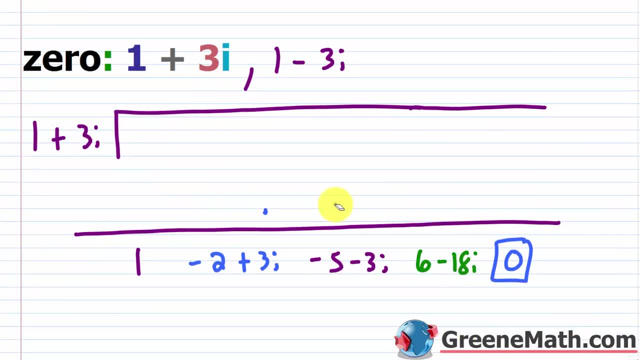 just going to use that. I'm going to erase this. I'm just going to take these guys. Okay, So I'm going to take my one. I'm going to take my negative. two plus three, i I'm going to take my negative. 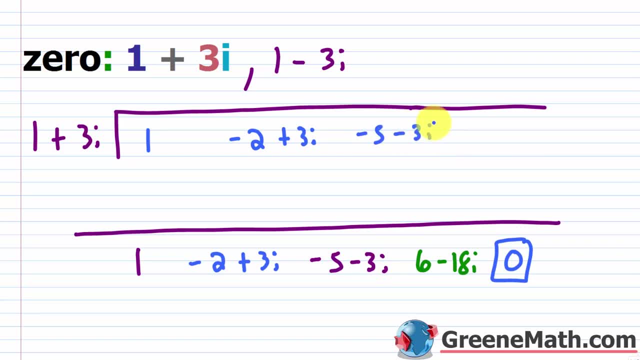 five- Let me put that as a minus. So minus three i, And then I'm going to take my six minus 18 i. So what we're going to do is now take the other zero, the one minus three i, because we know that's. 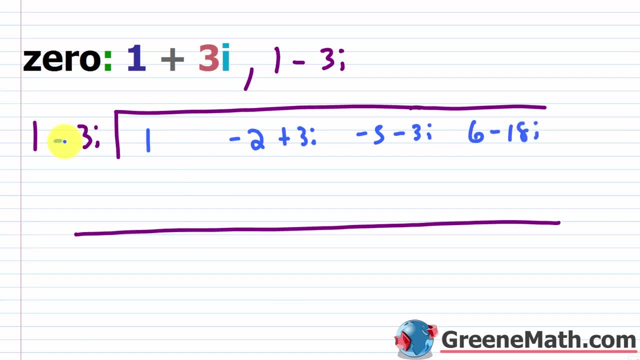 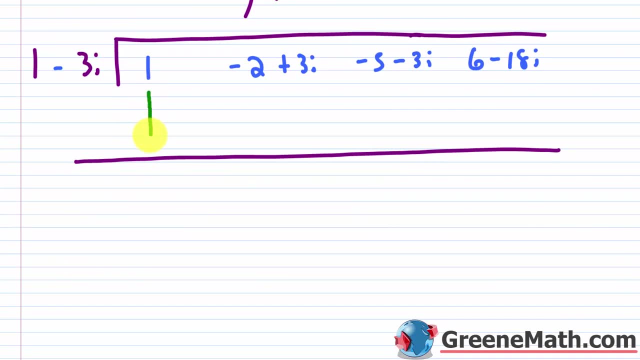 a zero And basically, when I take this quotient and divide it by this, I'm going to have a quadratic that I can then solve again with the quadratic formula or factoring or something like that, And I'll have all my zeros. Okay, So let's bring this down and say we have a one. So again, 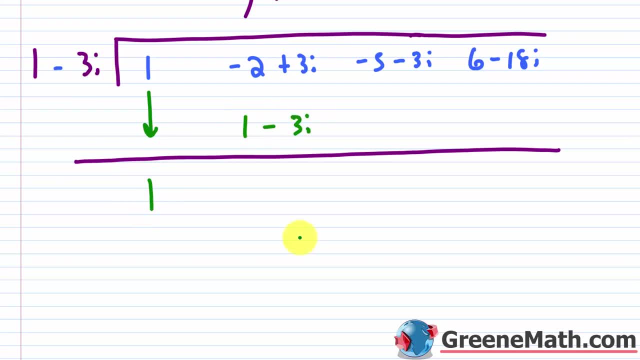 one minus three, i times one would be one minus three i. Okay. So when we add these you've got negative two plus one, which is negative one, And then positive three, i, which is negative. one minus three i is zero. Okay. So it's just negative one. Then one minus three, i times negative one. 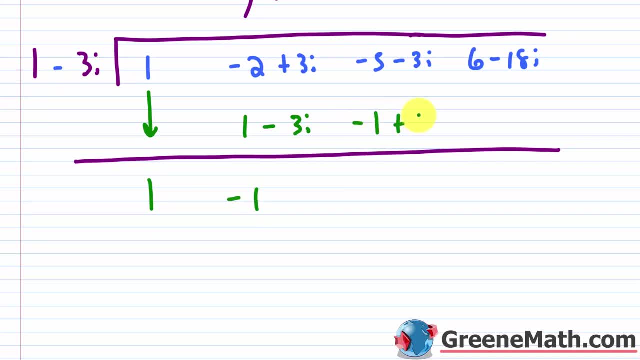 just change the sign of everything. So this would be negative one and then plus three, i, Okay. We add negative five plus negative one, or negative five minus one is negative six, Negative three: i plus three, i, that's zero, Okay. So now, lastly, we have one minus three, i times negative six. 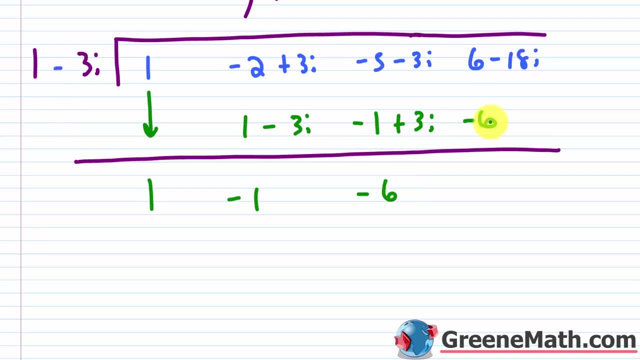 Again, I can just multiply each term by negative six. So this would be negative six And this would be plus 18 i. So again, we knew this was a zero. So we're going to take this: one minus three, i- zero. So this comes out to be zero, exactly, Okay, And these would be the coefficients for 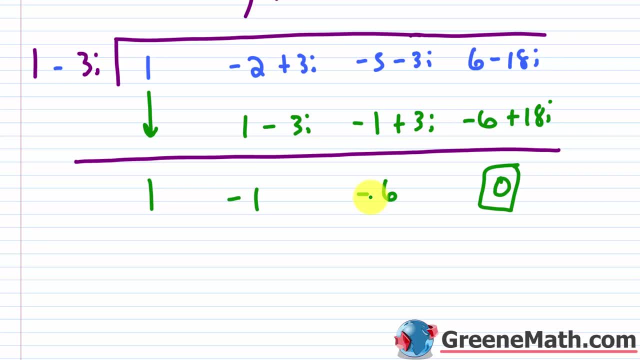 your polynomial function. Okay, That's your quotient. Now this is going to be of degree two. now We started with a fourth degree. We did one synthetic division, So it was a third degree. Now we did another one, So it's a second degree. So this guy is going to be the coefficient for x. 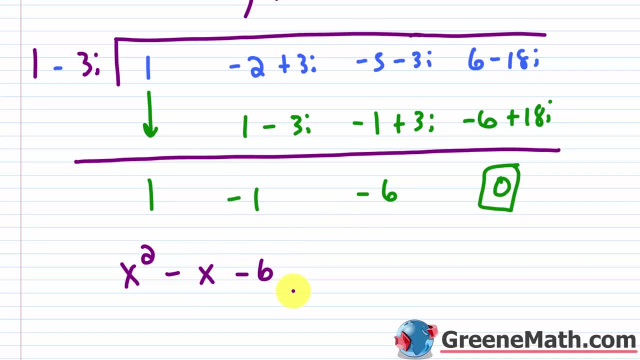 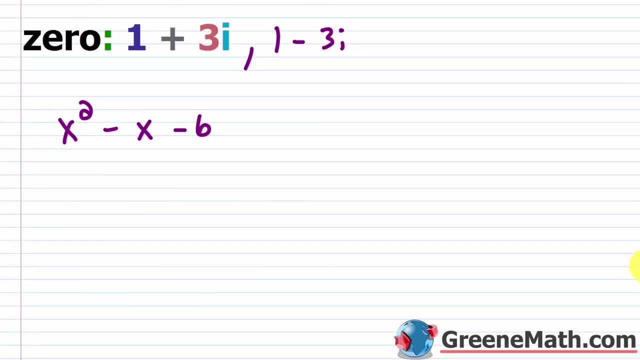 squared, Then this is x to the first power, Then this is your constant term. Okay, So this guy right here is what we're looking for. So I'll drag this up here and we'll come here and we'll just say, okay, where does this guy equal zero? Okay, And we can solve this. 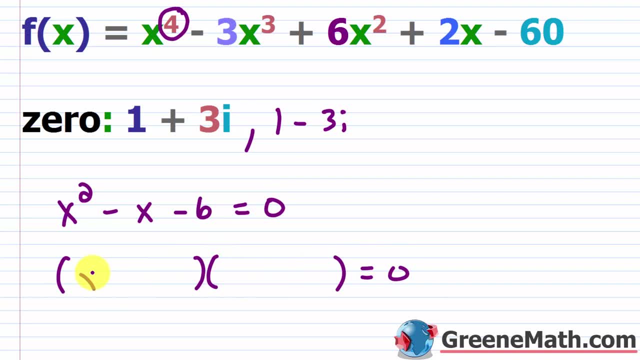 with factoring. Put an x here and an x here. Give me two integers that sum to negative one and give me a product of negative six. Well, you could do negative three and positive two. You could do negative three and positive two. So, obviously, if you solve this, you would get x. 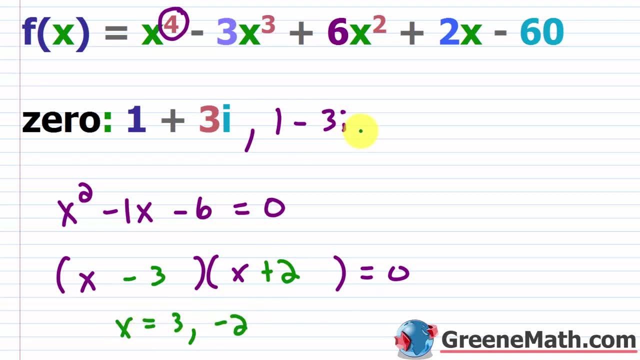 is equal to three or negative two. So I can just add this to my list here And say that another zero would be three and another one would be negative two. I know I said zero here. This should be zeros, But when I started it was singular. We just had one. So 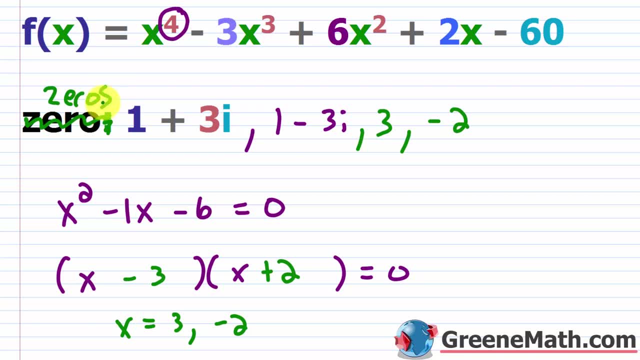 let me just mark this out and say these are the zeros. Okay, Plural, So we have our one plus three i, which was given to us, our one minus three i, which is the conjugate. Then we have three and negative two which we found.